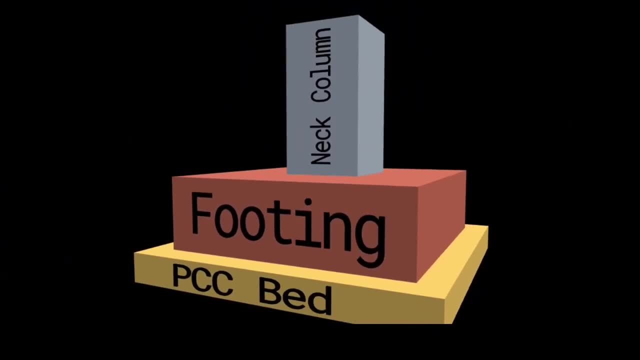 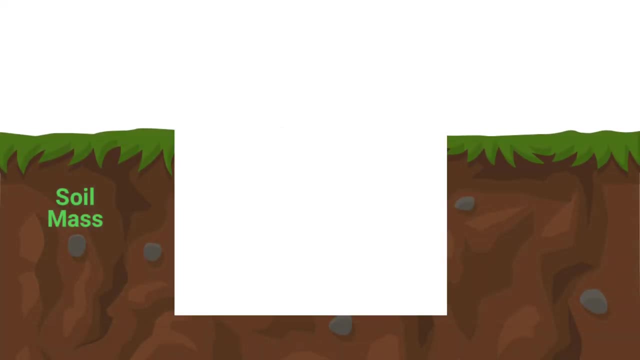 To do the calculation for footing at the construction site, we need to follow some basic steps. The first step is to do the excavation process, in which we need to dig a bit for the foundation. After leveling the bed properly, an antitermite powder is applied on the bed surface. 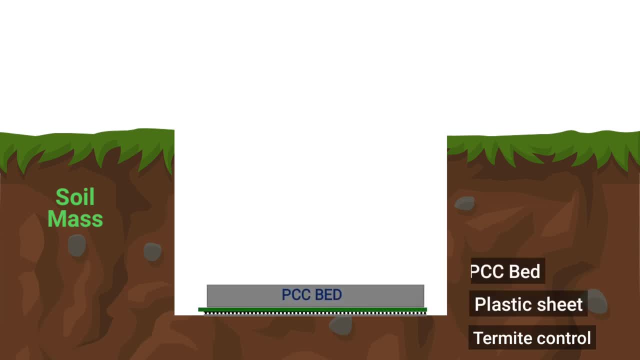 which is followed by a polythene covering on which PCC bed is laid. The polythene covering acts as a barrier between concrete and soil mass. If we don't apply the polythene covering, the soil would absorb the water from concrete. As a result, the concrete would lose its strength. 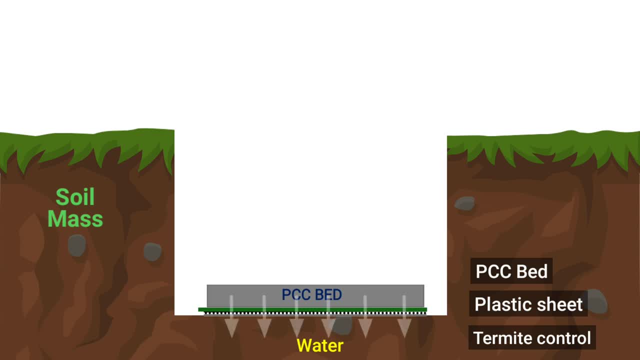 So to maintain the strength of concrete, polythene sheets are laid before the application of PCC bed. After laying the PCC bed, the next step is to cast the footing, followed by raising the column above the footing. The surfaces of the column and footing are coated by bitumen paint. 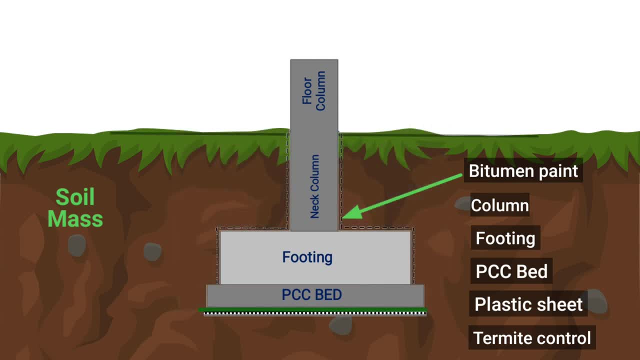 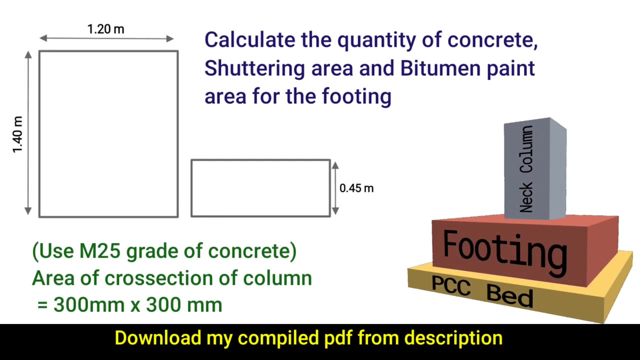 up to the ground level. The purpose of application of this paint is to protect the material of column and footing, that is, concrete and Steel, from the moisture content present in the backfill, The __________. Let us take an example in which we have a footing of length 1.2 meter, width 1.4 meters. 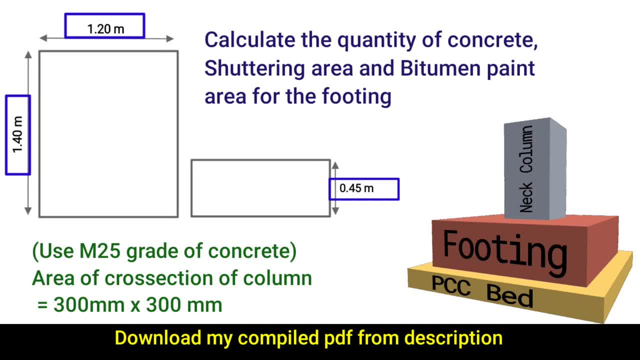 and the depth of footing b equal to 0.45 meter. ____________. The grade of concrete used in this footing is M25 and the area of cross section of the column about this footing is 300mmX23 inches. fork design of a concrete mat is now to prevent that of powder upon that wood passed between the backfill and backfill HalloweenIl. 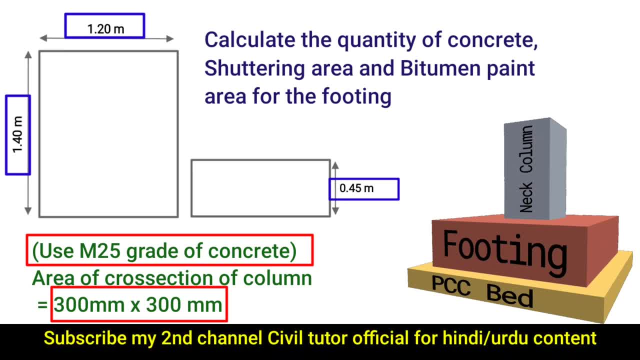 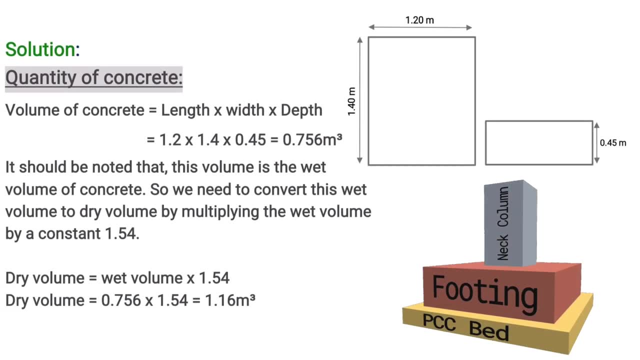 into 300 mm. Suppose we need to calculate the quantity of concrete, the shuttering area and the bitumen paint area of this footing. I will show you the calculation of its PCC bed in my next lecture. To calculate the quantity of concrete we 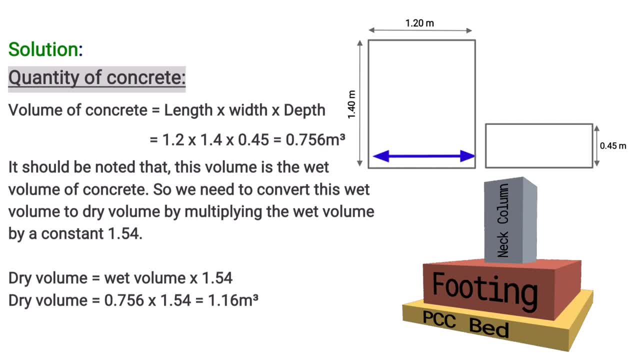 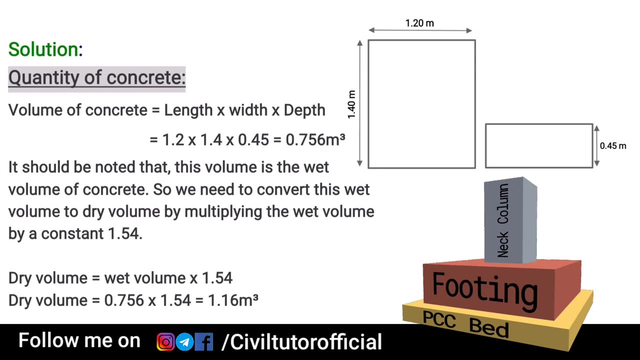 need to calculate the volume of concrete, which will be equal to length of footing into width of footing, into depth of footing. On substituting these values, we will get the volume of concrete equal to zero point seven, five, six meter cube. It should be noted that this volume is the wet volume of concrete, so we need to. 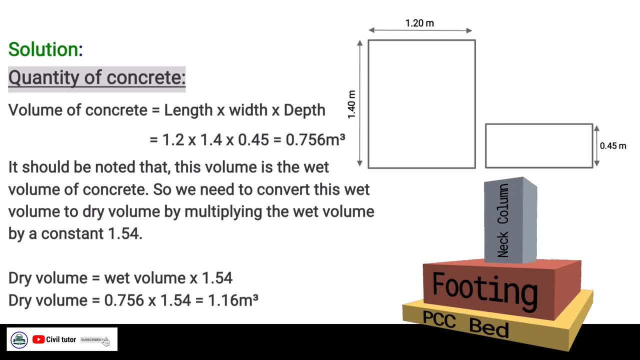 convert this wet volume to dry volume by multiplying it with conversion factor 1.54.. So dry volume will be equal to wet volume into 1.54.. As wet volume is already calculated as 0.75, 6 meter cube, so on substituting these values we will: 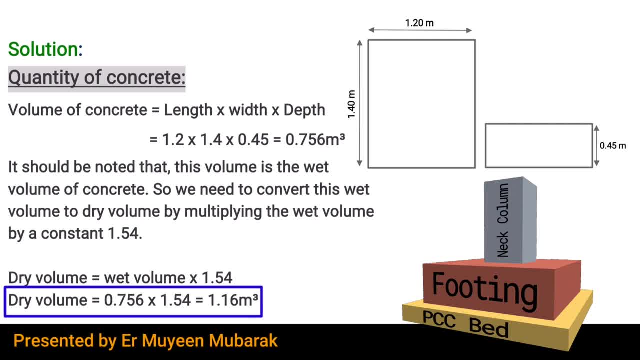 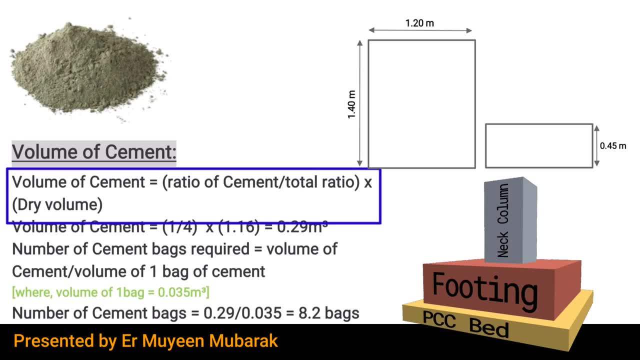 get the value of dry volume equal to 1.16 meter cube. now we need to calculate the volume of cement. volume of cement is equal to ratio of cement upon total ratio into dry volume. ratio of cement used in m25 grade of concrete is 1 total. 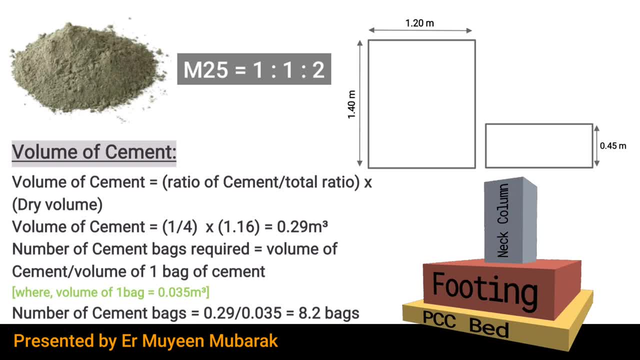 ratio will be equal to ratio of cement plus ratio of sand plus ratio of aggregate, which is 1 is to 1, is to 2, so total ratio will be equal to 4, and dry volume is calculated as 1.16 meter cube. so on substituting these values, we will: 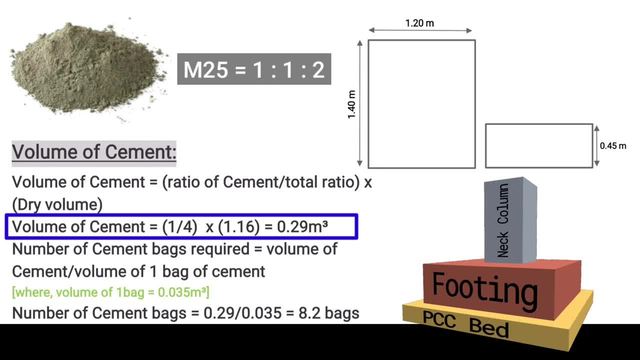 get the volume of cement equal to 0.29 meter cube, number of cement bags will be equal to volume of cement upon volume of one bag of cement. volume of cement is calculated as 0.29 meter cube and volume of one bag of cement is equal to. 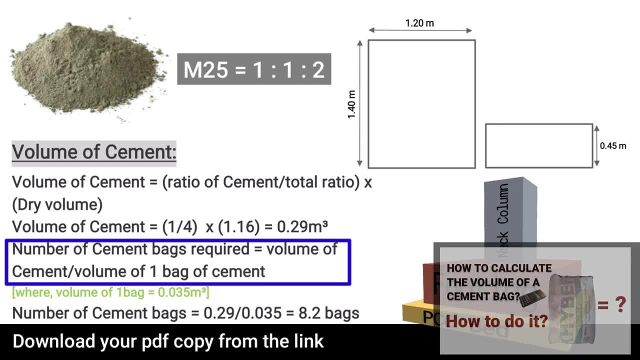 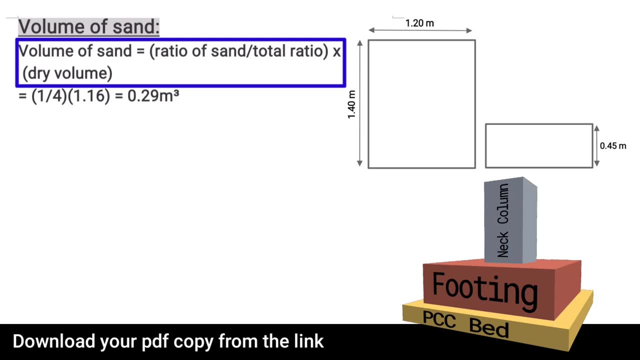 0.035 meter cube. so on substituting these values, we will get the number of cement bags equal to eight point two bags. now we need to calculate the volume of sand. volume of sand will be equal to ratio of sand upon total ratio into dry volume. as the ratio of sand used is one, total ratio is: 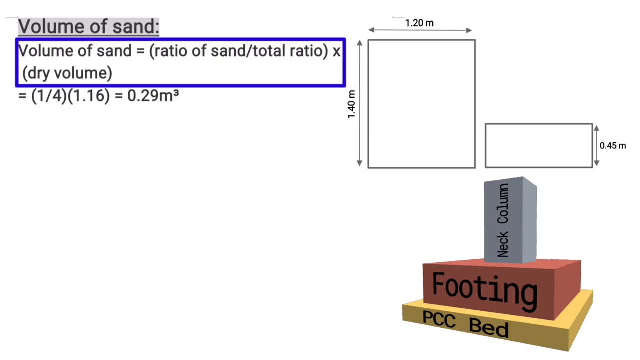 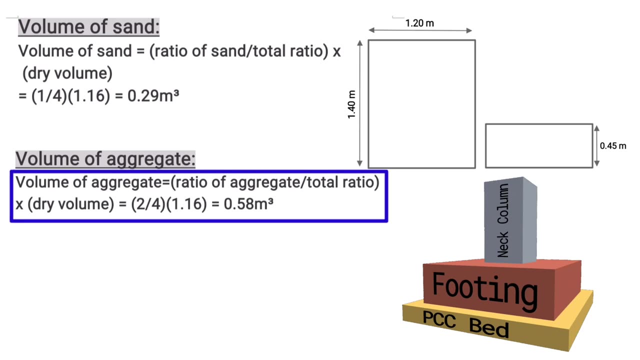 4, and dry volume is already calculated as 1.16.. So on substituting these values, we will get the volume of sand equal to 0.29 m3.. Volume of aggregates will be equal to ratio of aggregate upon total ratio into dry volume. 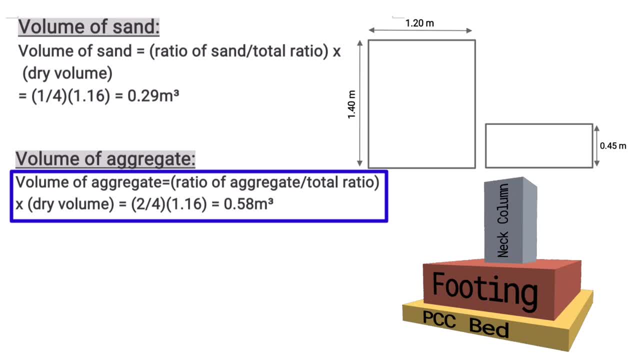 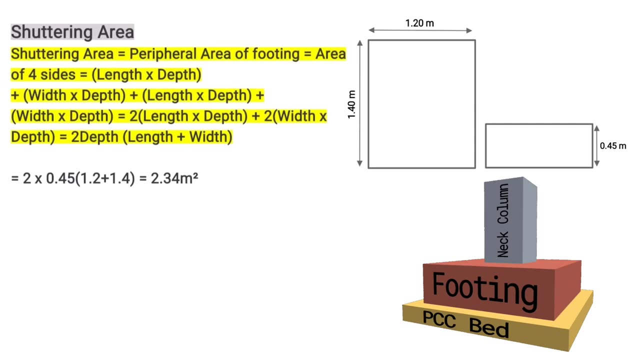 As the ratio of aggregate used is 2, total ratio is 4 and dry volume 1.16 m3.. So, on substituting these values, we will get the volume of aggregate equal to 0.58 m3.. Now we need to calculate the shuttering area, which will be equal to peripheral area of